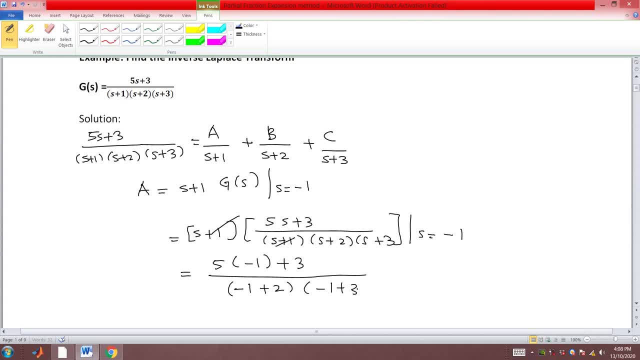 1 plus 3,, which is equal to minus 1.. So now a equal minus 1.. How about b? Okay, b 1 equal s plus 2 times gs s equal minus 2, yeah, So s plus 2 times 5s plus 3 over. 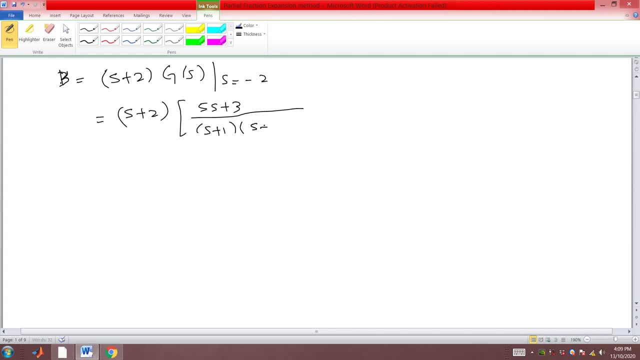 s plus 1. times s plus 2. times s plus 3. s equal minus 2, yeah, So cancel here, and here we can get 5s plus 3 over s plus 1. times s plus 3 s equal minus 2. 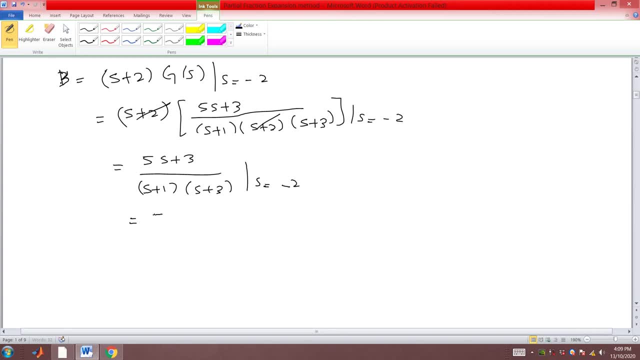 so 5 minus 2 plus 3 over minus 2 plus 1 minus 2 plus 3, which is equal to 7. so b equal 7, b equal 7. now we need to find c, c equal s plus 3 times d. 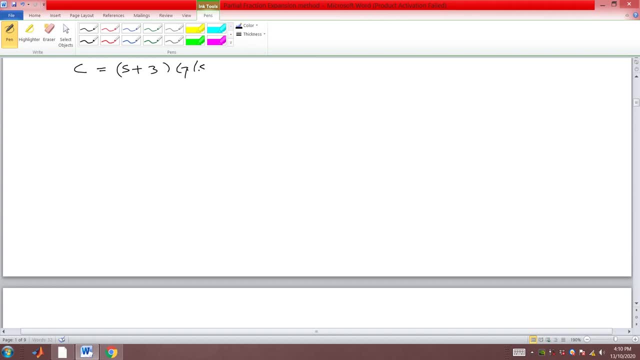 s equal minus 3, so s plus 3 times 5s plus 3 over s plus 1 s plus 2 times s plus 3 s equal minus 3. so this one cancel each other. so left is 5, so substitute minus 3. 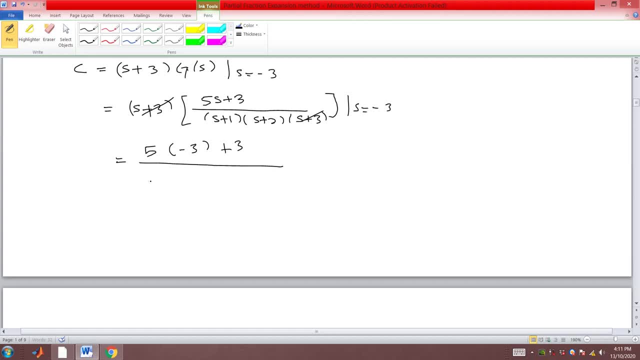 plus 3, so s plus 3 over minus 3 plus 1. minus 3 plus 2. Ok, that's alright. so which is equal to minus 6, so c equals minus 6. so c equal minus 6, so c equals minus 6. 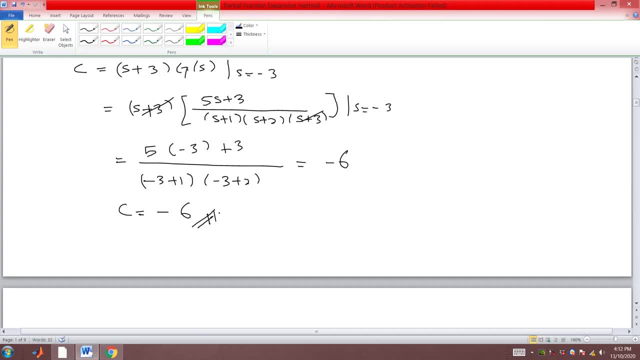 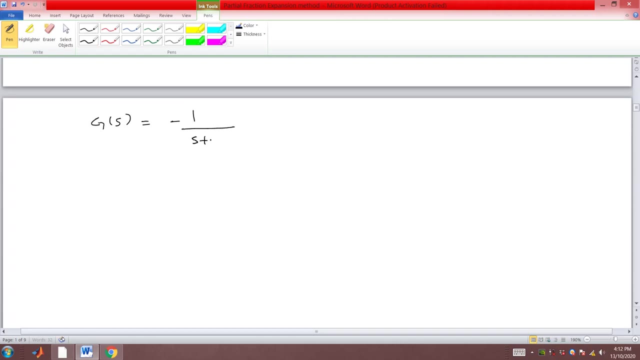 so c equal minus 6. so c equal minus 6. So now gs equal minus 1 over s plus 1 plus 7 over s plus 2 minus 6 over s plus 3.. So we need to inverse the plus. 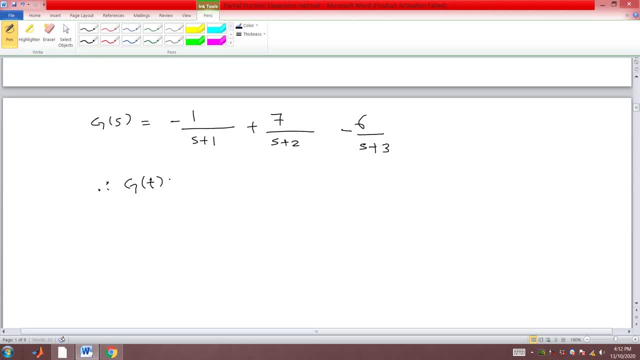 So gt equal minus e minus t, ut plus 7 e minus 2t, minus 6 e power of minus 3t. So this is also ut right, This is also ut. Okay, We need to group. We need to group it. 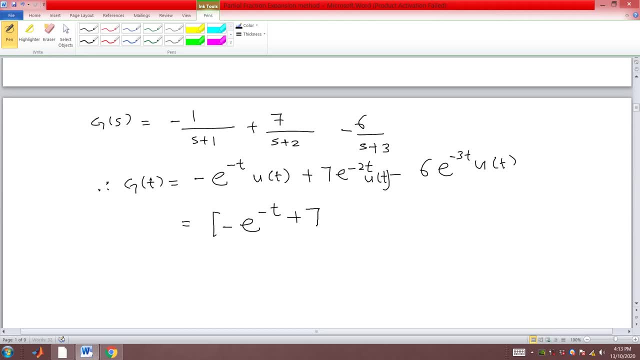 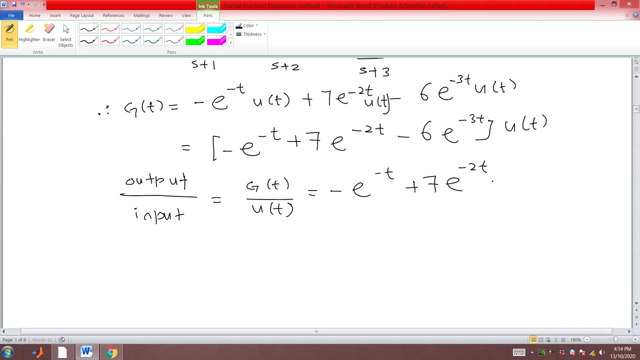 Minus e t plus 7 e minus 2t, minus 6 e power of minus 3t. So this one, Of course it is gtf, Okay, Okay. So output Over input, yeah, equal gt over ut, which is minus e minus t, plus 7 e minus 2t, minus 6 e power of minus 3t.